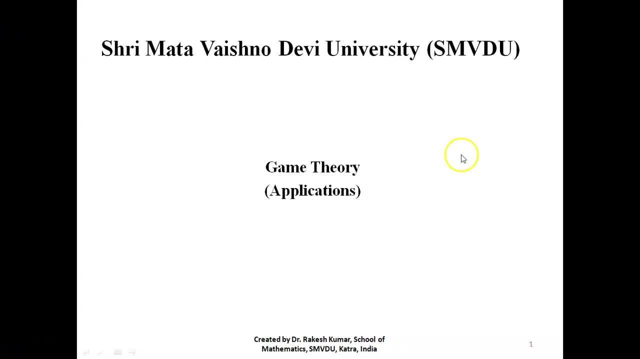 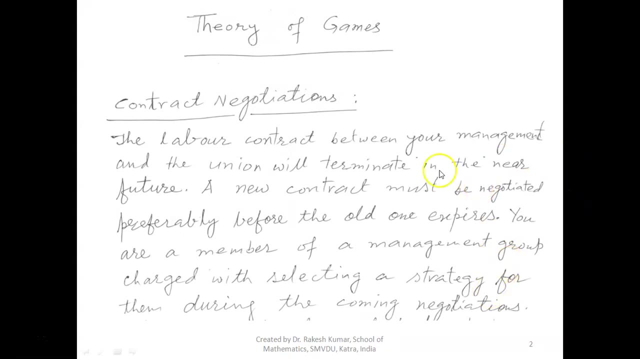 Hello, today we will learn some applications of game theory. First situation that we will take up, that is contract negotiations. The labor contract between your management and the union will terminate in the near future. A new contract must be negotiated, preferably before the old one. 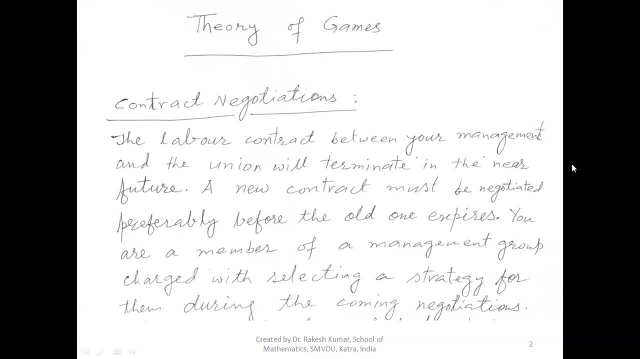 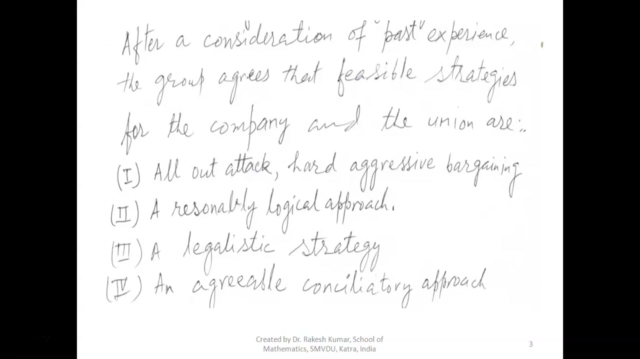 expires, You are a member of management group charged with selecting a strategy for them during the coming negotiations. After a consideration of past experience, the group agrees that feasible strategies for the company and the union are. So in order to negotiate a new contract, both the parties agree that following may be the feasible: 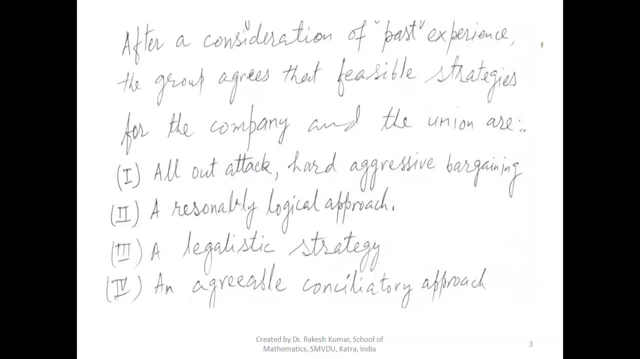 strategies. Number one: strategy number one: all out attack, that is, hard aggressive bargaining. Second, a reasonably logical approach. Third, a legalistic strategy. and fourth, an agreeable conciliatory approach. So these are the four possible strategies which will be considered by the company as well as the union. 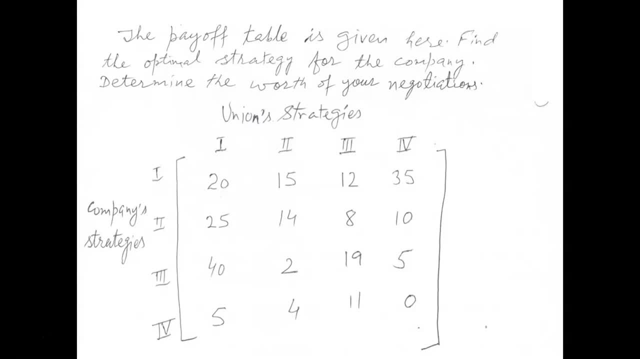 The payoff table is given here. Find the optimal strategy for the company. Determine the worth of your negotiations. So, from the past experience, this is the payoff matrix to the company: Company strategies: row wise 1,, 2,, 3, 4 and union strategies, column wise 1,, 2,, 3, 4.. 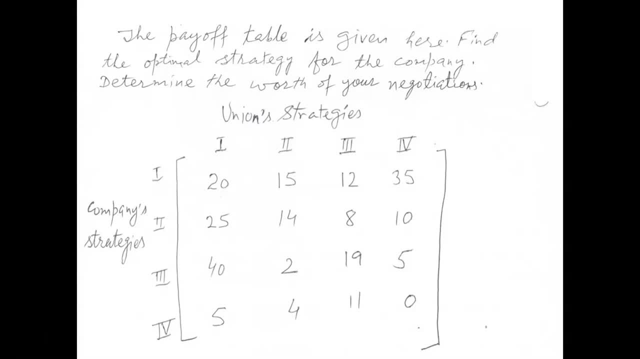 So if company chooses strategy 1 and union chooses strategy 1, so there will be a payoff of 20 units to company And similarly we can interpret all other payoff values in this payoff matrix. Now what is the question? The question was: find the optimal strategy for the company as well as the optimal strategies for the union. 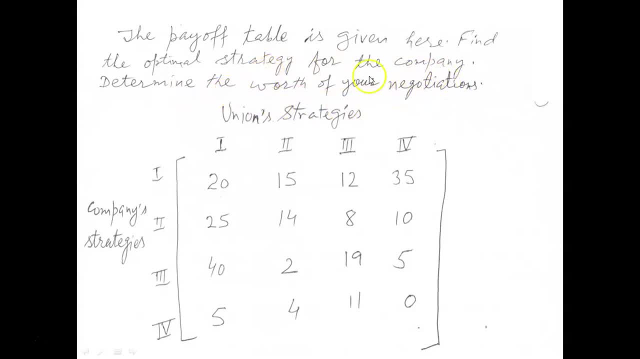 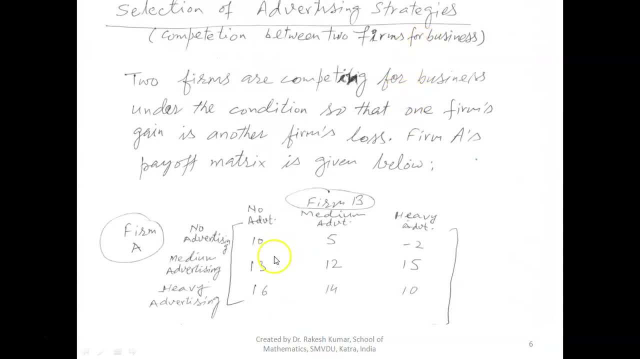 So, in order to answer this type of situation, decision making framework game theory helps us. So, in order to answer this type of situation, decision making framework game theory helps us. business okay. so there could be various kind of no games- business games okay.